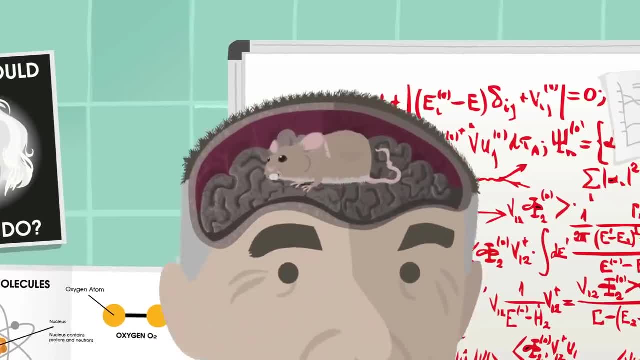 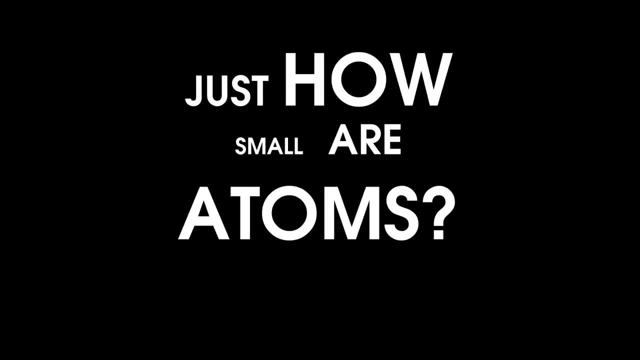 haven't ever thought about how small atoms really are? Well, the answer is that they are really, really, really small. So you ask: just how small are atoms? Well, to understand this, let's ask this question: How many atoms are in a grapefruit? Well, let's assume that the 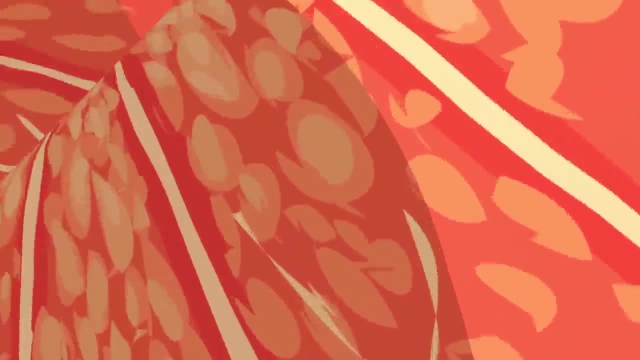 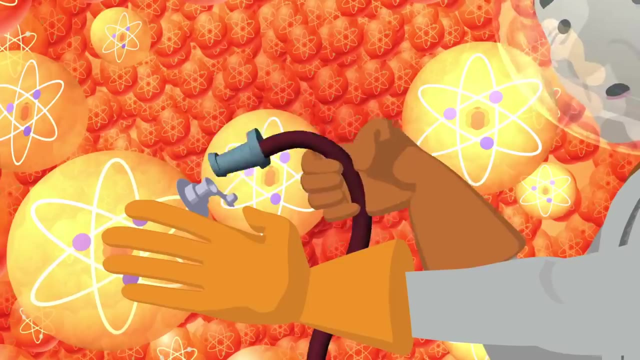 grapefruit is made up of only nitrogen atoms, which isn't at all true, but there are nitrogen atoms in a grapefruit. Well, to help you visualize this, let's blow up each of the atoms to the size of a blueberry, And then how big would the grapefruit have to be? 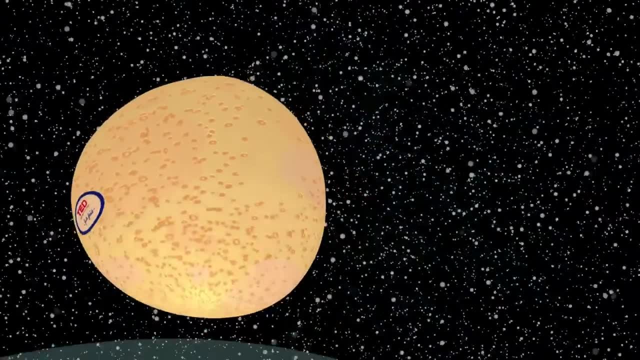 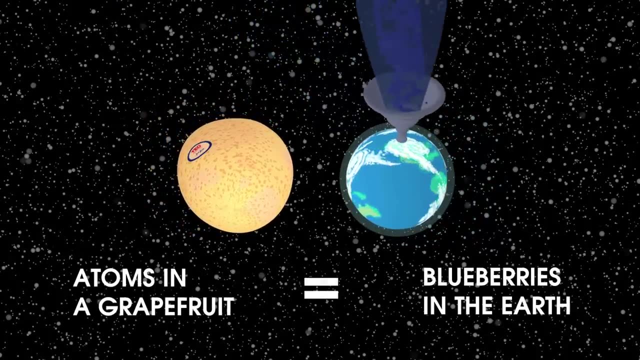 It would have to be the same size of- well, actually, the Earth. That's crazy. You mean to say that if I filled the Earth with blueberries, I would have the same number of nitrogen atoms as a grapefruit. That's right. So how big is the atom? Well, it's really, really, really really. 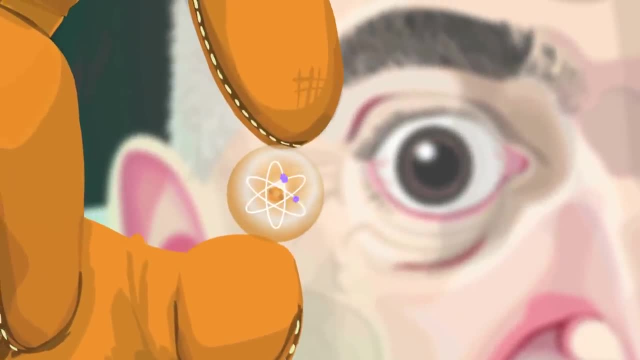 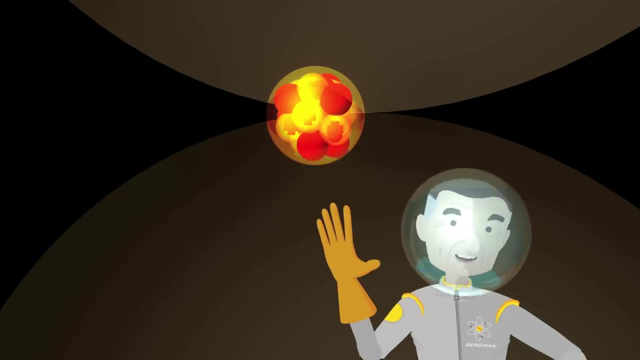 small, And you know what. It gets even more crazy. Let's now look inside of each atom. That's the blueberry right. What do you see there? In the center of the atom is something called the nucleus, which contains protons and neutrons, And on the outside you'd see electrons. So how big is the 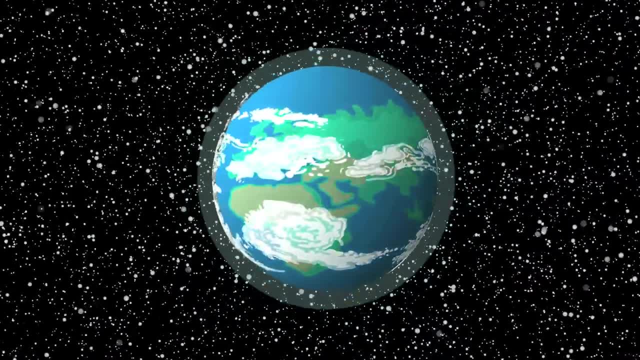 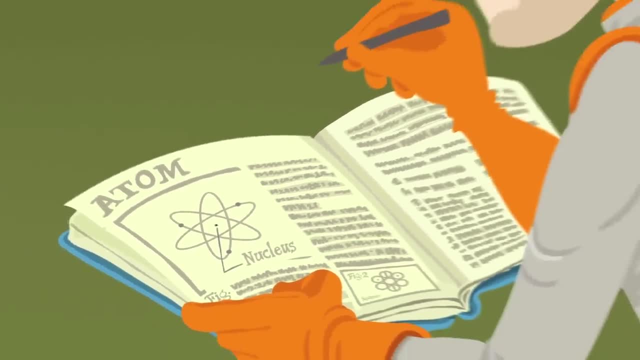 nucleus. Well, if atoms are like blueberries in the Earth, how big would the nucleus be? You might remember the old pictures of the atom from your science class where you saw this tiny dot on the page with an arrow pointing to the nucleus. Well, those pictures, well, they're not drawn to scale. 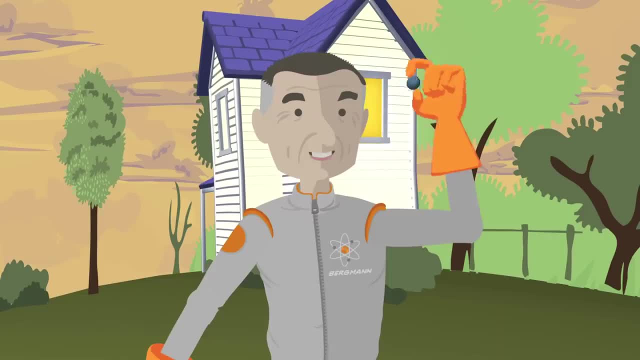 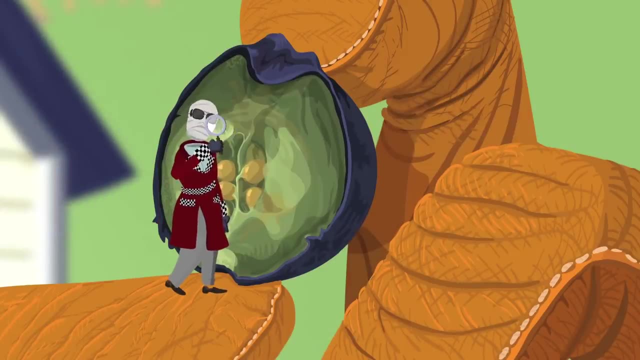 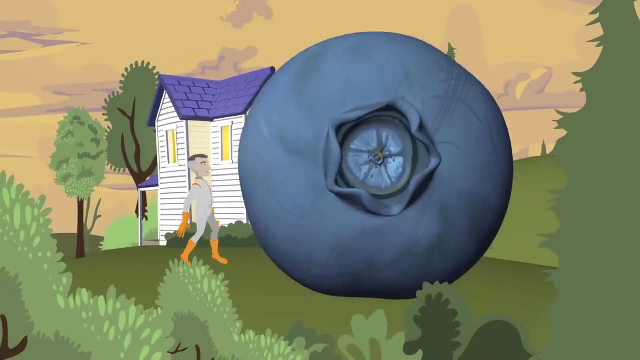 so they're kind of wrong. So how big is the nucleus? So if you popped open the blueberry and were searching for the nucleus, you know what? It would be invisible, It's too small to see. Okay, let's blow up the atom, the blueberry, to the size of a house. 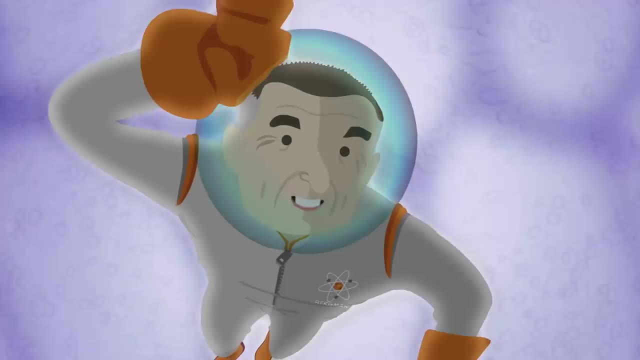 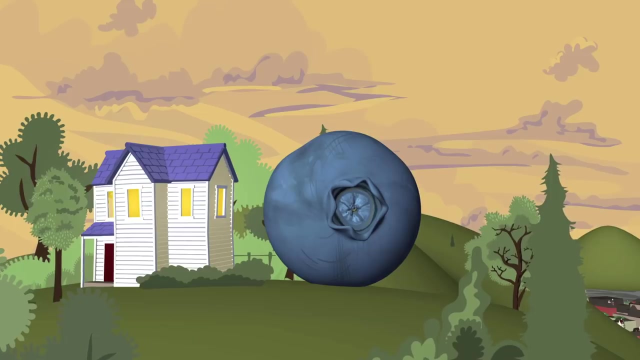 So imagine a ball that is as tall as a two-story house. Let's look for the nucleus in the center of the atom, And you know what? It would just barely be visible. So to get our minds wrapped around how big the nucleus is, we need to blow up the blueberry up to the size of a football stadium. 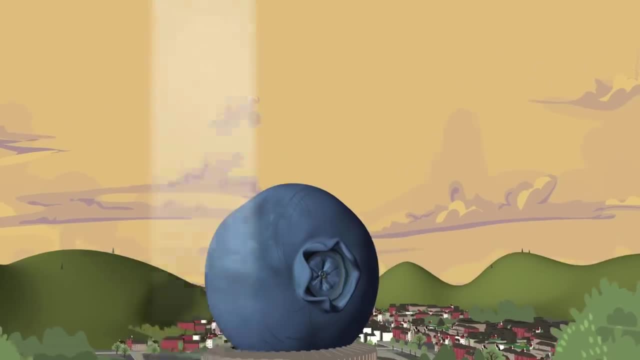 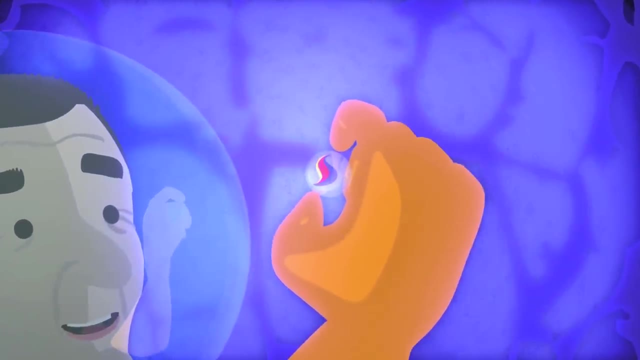 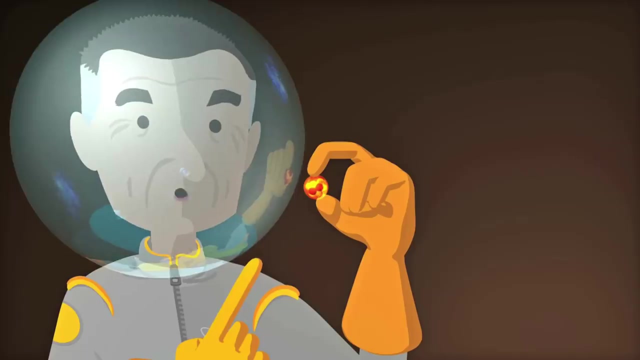 So imagine a ball the size of a football stadium And right, smack dab in the center of the atom, the nucleus, And you could see it, And it would be the size of a small marble. And there's more, If I haven't blown your mind by now. let's consider the atom some more. It contains protons, neutrons. 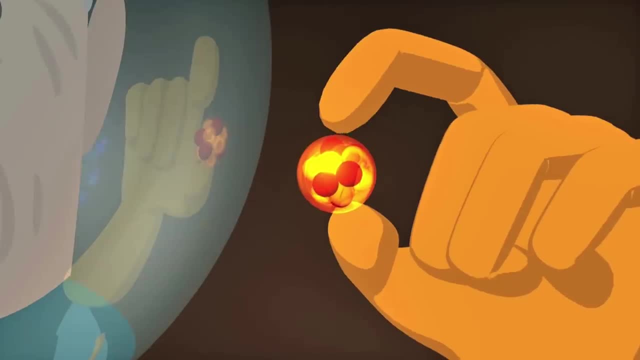 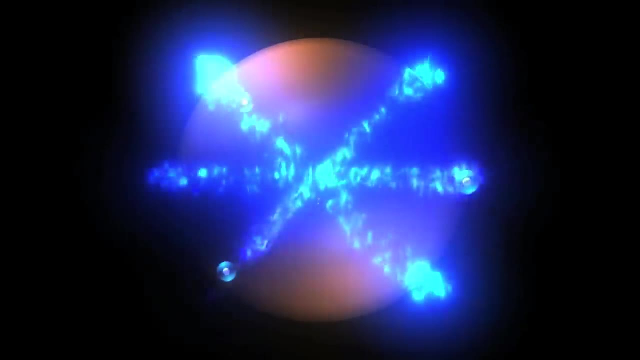 and electrons. The protons and neutrons live inside of the nucleus and contain almost all of the mass of the atom. Way on the edge are the electrons. So if an atom is like a ball the size of a football stadium, with a nucleus in the center and the electrons on the edge, what is in? 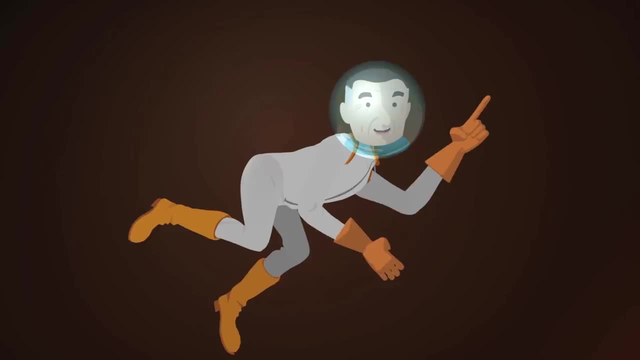 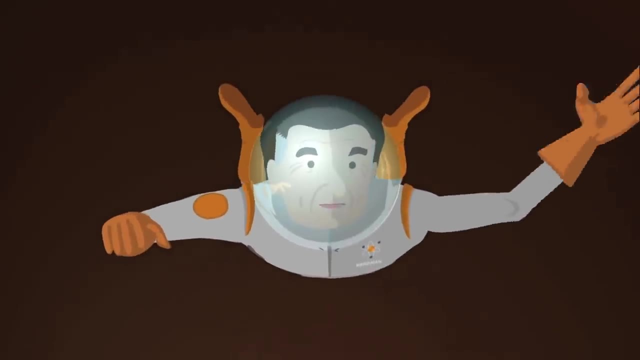 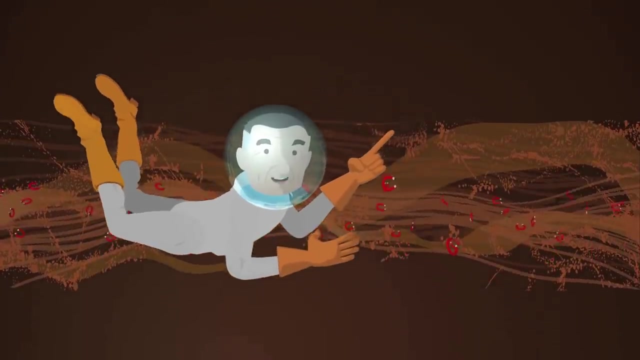 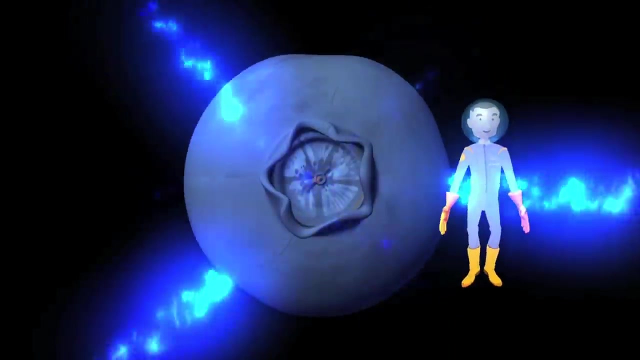 between the nucleus and the electrons. That's right: Empty. Between the nucleus and the electrons. there are vast regions of empty space. Now, technically, there are some electromagnetic fields, but in terms of stuff, matter, it is empty. Remember, this vast region of empty space is inside the blueberry, which is inside the earth. 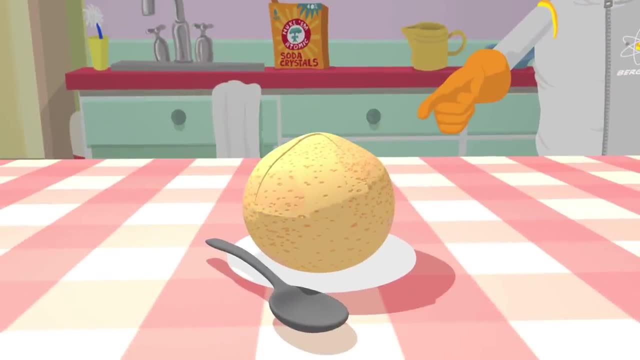 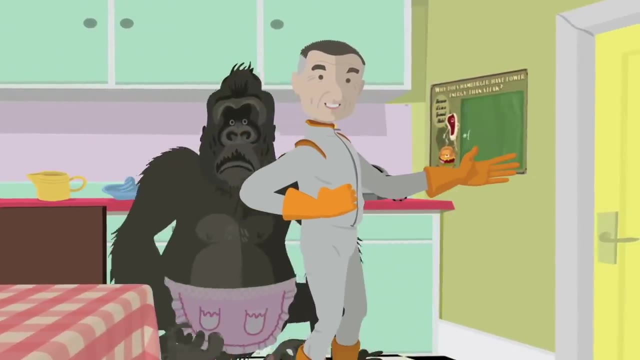 which really are the atoms in the grapefruit. Okay, one more thing, if I can even get more bizarre, Since virtually all of the mass of an atom is inside the blueberry. what is inside the nucleus? Now, there is some amount of mass in the electrons, but most of it is in the nucleus. 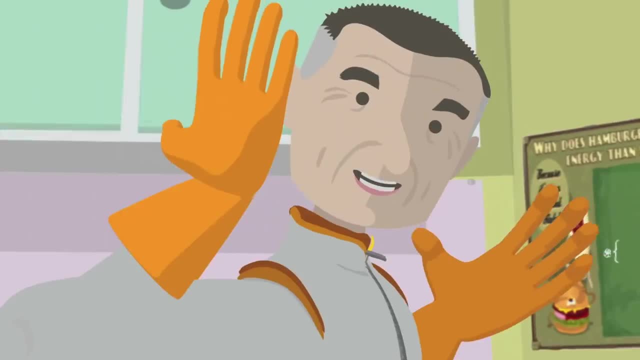 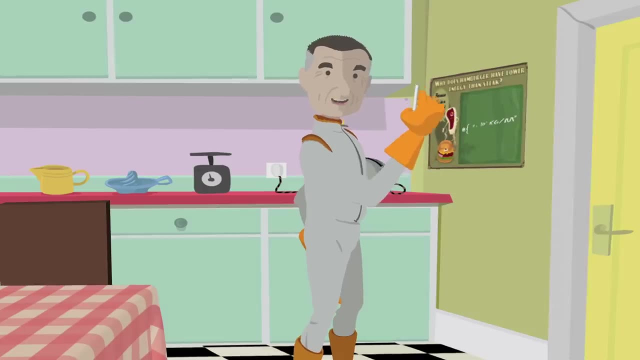 How dense is the nucleus? Well, the answer is crazy. The density of a typical nucleus is 4 times 10 to the 17th kilogram per meter cubed. But that's hard to visualize. Okay, I'll put it in. English units, 2.5 times 10 to the 16th pounds per cubic feet. Okay, that's still kind of hard to figure. Okay, here's what I want you to do: Make a box that is one foot tall and one foot. 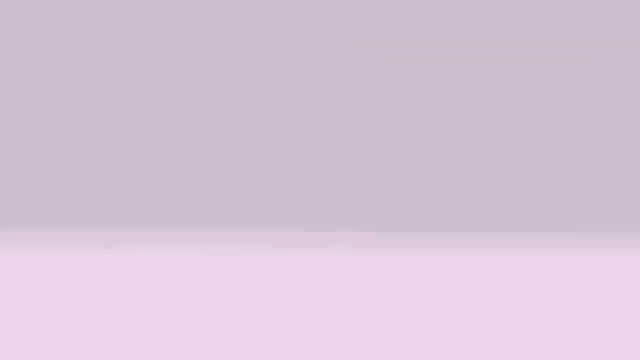 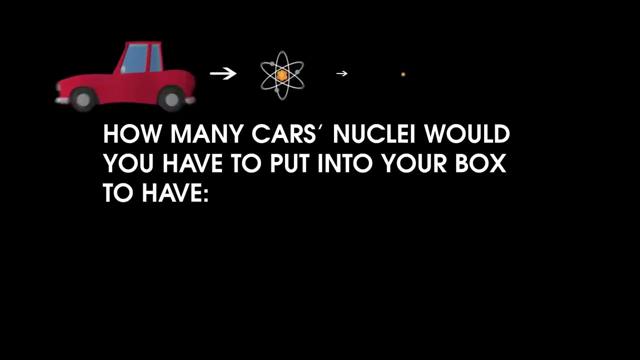 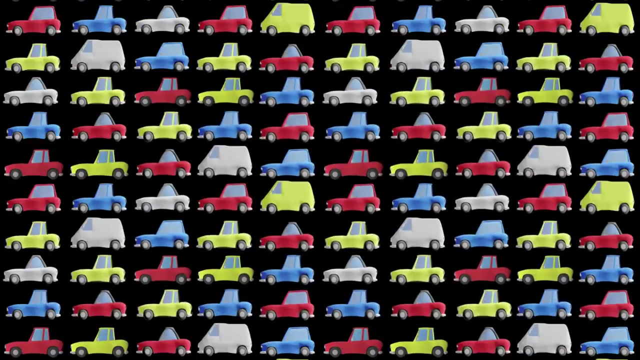 by one foot, by one foot And let's go and grab all of the nuclei from a typical car. Now, cars on average weigh two tons. How many cars' nuclei would you have to put into the box to have your one-foot box have the same density of a nucleus? Is it one car Two? How about a hundred? Nope, 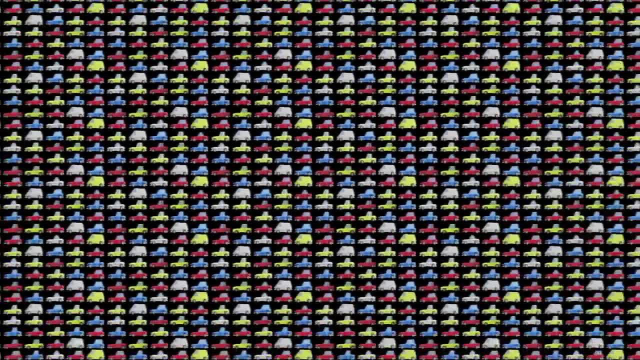 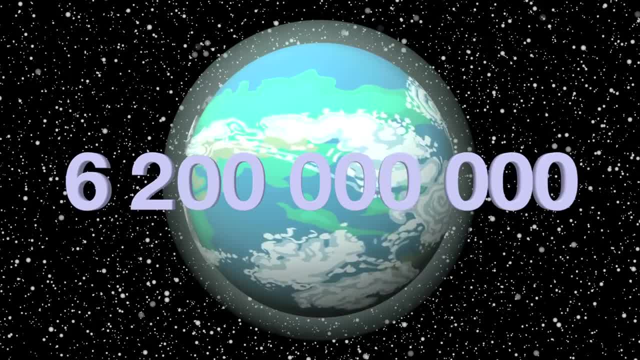 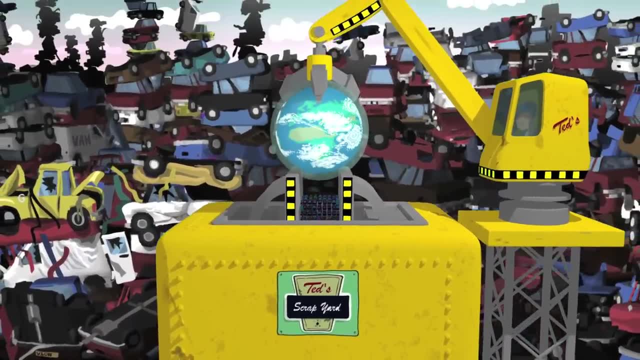 nope and nope. The answer is much bigger. It is 6.2 billion. That is almost equal to the number of people in the earth. So if everyone on the earth on average would own their own car and they don't- and we put all of those cars into your box. 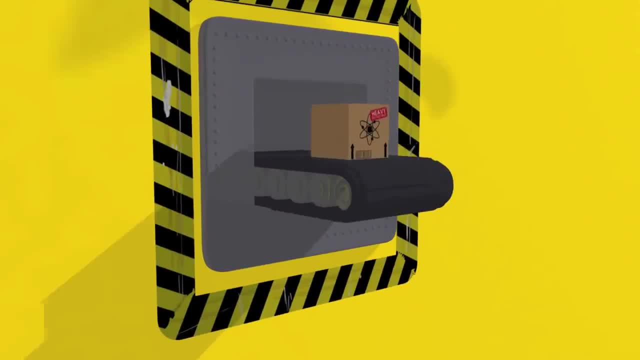 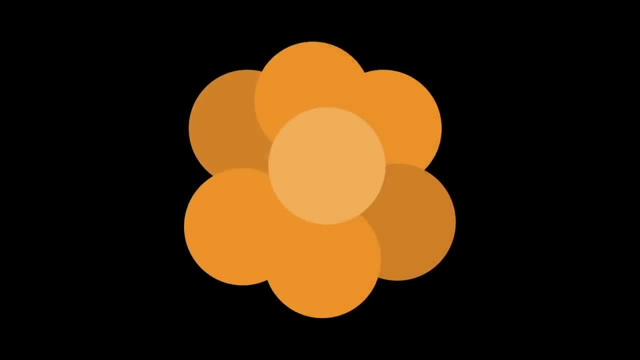 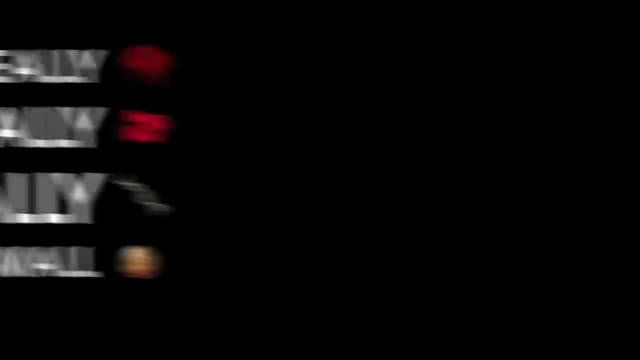 that would be about the density of a nucleus. So I'm saying that if you took every car in the world and put it in your one-foot box, it would have the density of one nucleus. Okay, let's review. The atom is really really, really small. Think atoms in a grapefruit, like blueberries in. 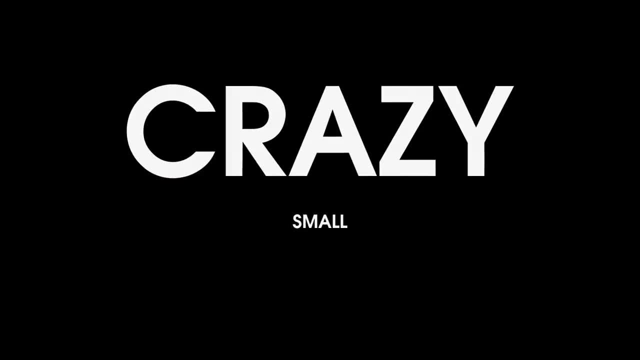 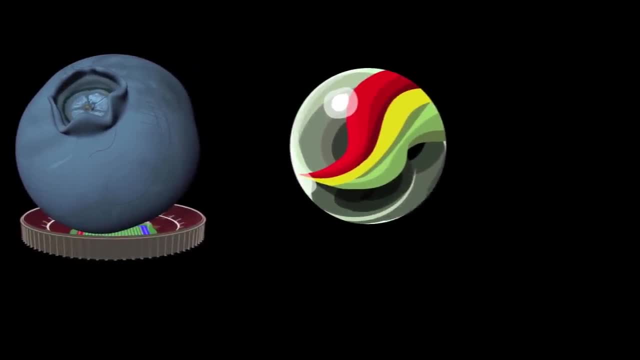 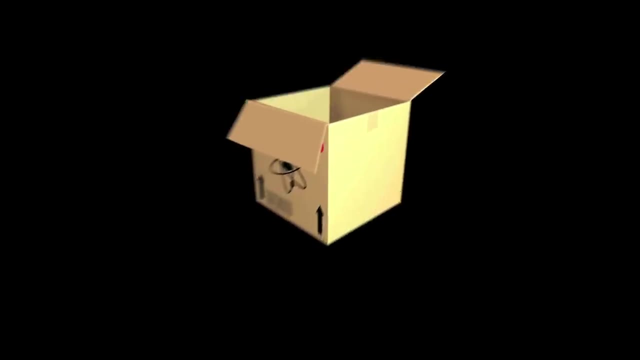 the earth. The nucleus is crazy small. Now look inside the blueberry and blow it up to the size of a football stadium, and now the nucleus is a marble in the middle. The atom is made up of vast regions of empty space. That's weird. The nucleus has a crazy high density. I'm thinking putting all those cars. 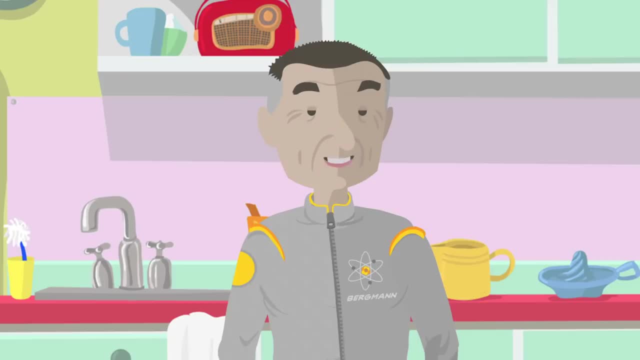 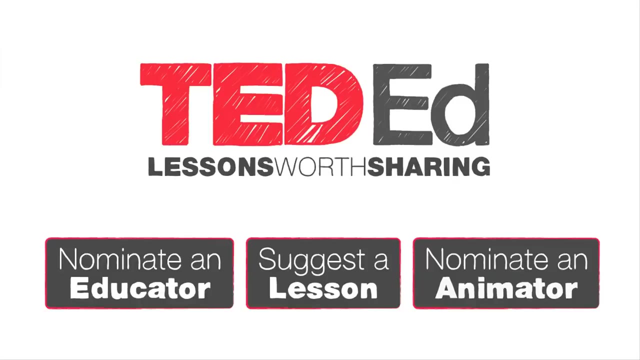 in your one-foot box. I think I'm tired. 1,200,000 people on this planet. There are only three of these cars in the universe, Right, I feel like they're mostly cars and some of them are car cars and some of them are cars. I don't know why. Oh, I don't know. I think it's probably the because they're so small. I don't think it's because they're small. So the nucleus is like a small car, but even larger. And they're big, small. Yeah, and I think they're too small to be counted as big cars. They're like small cars, but there's a lot of them, That's true, Yeah. Yeah, You're right, I don't know, There's a lot to be counted as big cars. 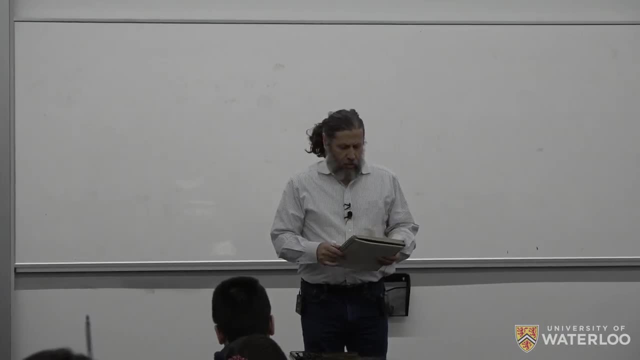 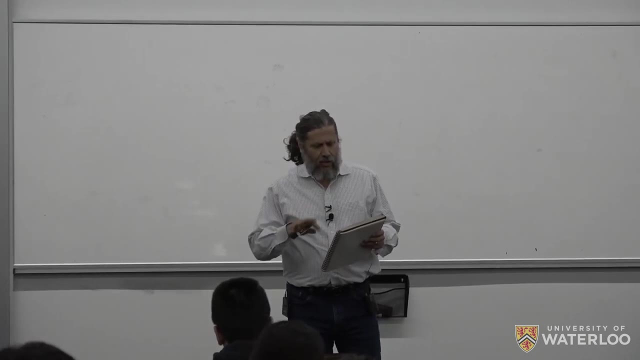 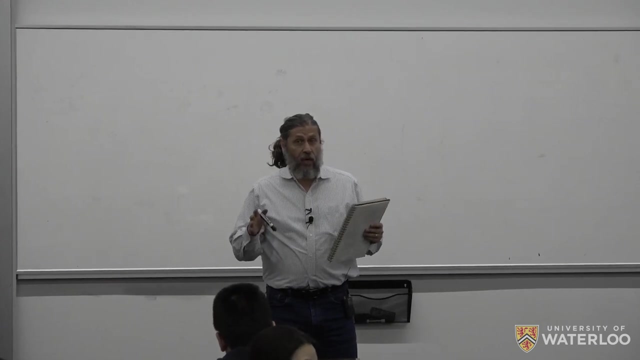 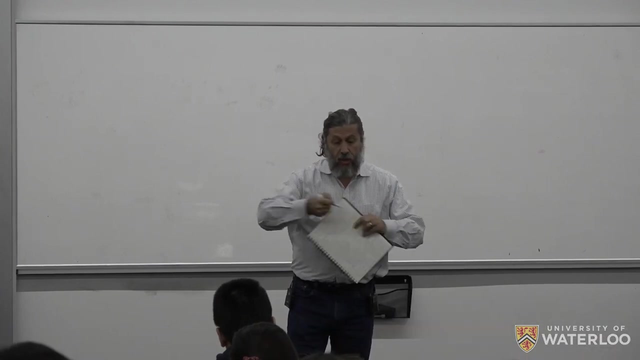 Okay, good afternoon everybody. So we talked a little bit about what people call fuzzy logic and we want to dedicate this lecture to, because it offers us one mechanism that we use a lot, which is inferencing- How can I use existing data to infer new knowledge? So we want to cover that today. Hopefully we get a good idea about it. 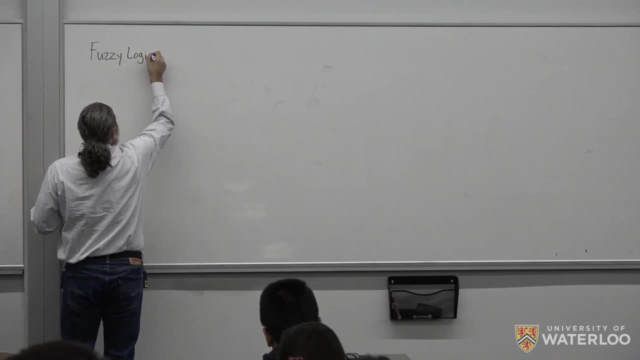 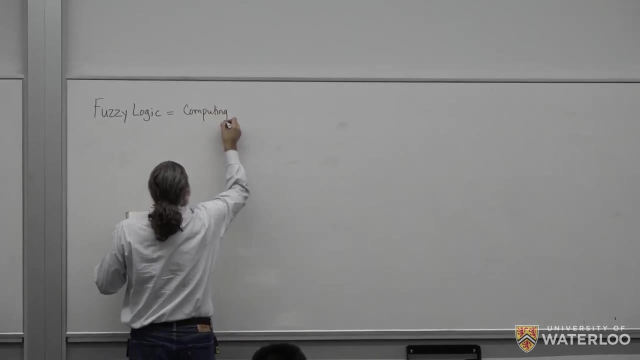 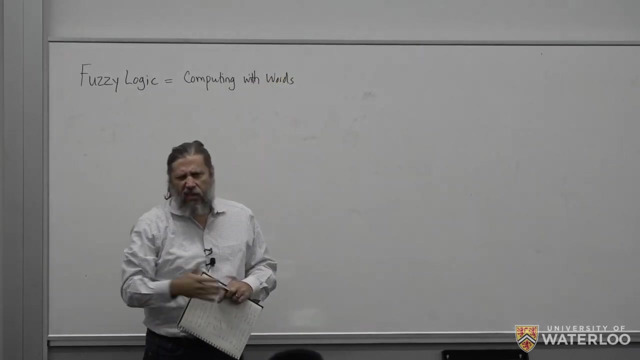 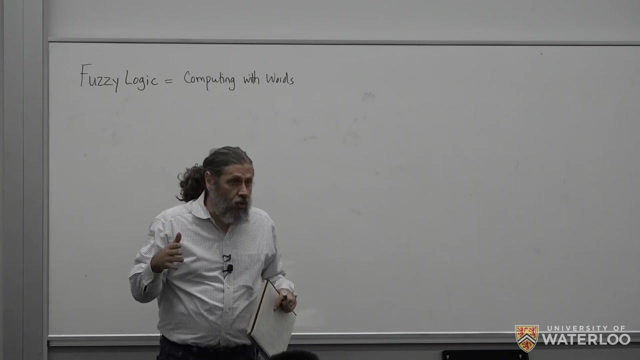 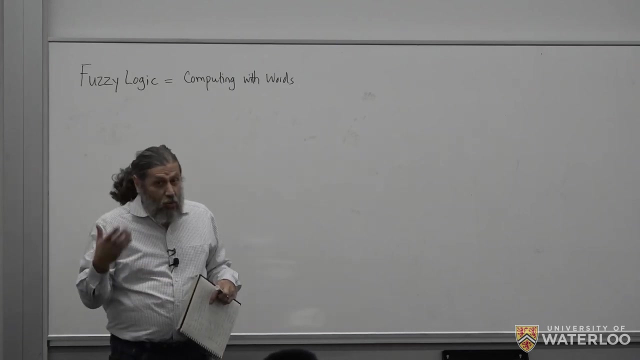 Fuzzy logic was supposed to be computing with words. I guess we are not there yet, mainly because our computers cannot process words. The natural language processing that we do with TFIDF and LSTM and all that are nice and good, But we are not processing really words. So processing words is a different thing. For 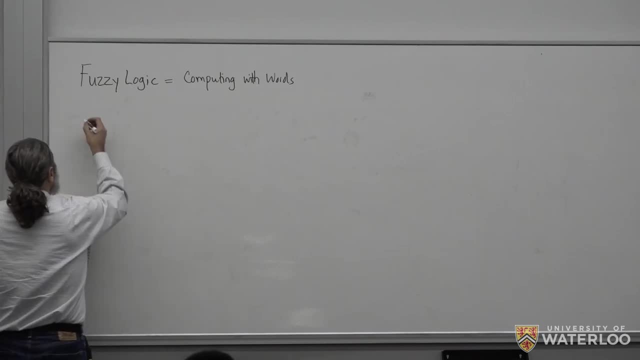 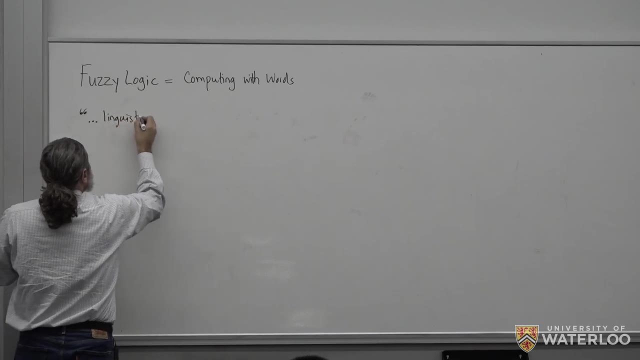 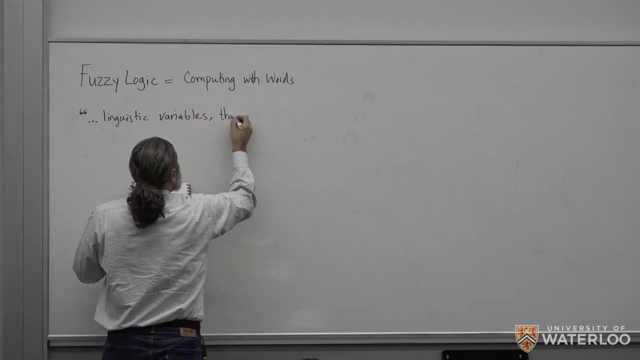 that you need special type of computers. We don't have those computers, because if you have those computers, you should be able to process linguistic variables. So that is, variables of the language. Okay, Okay, Okay, Okay, Okay Okay.